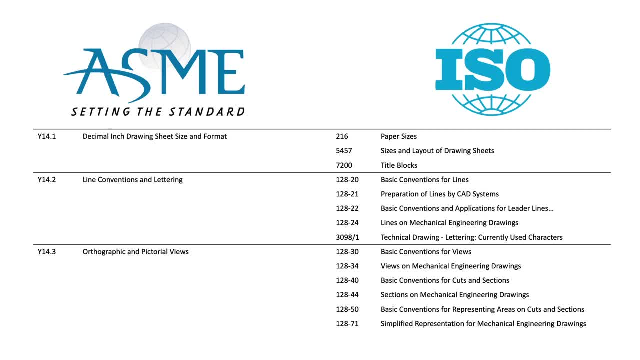 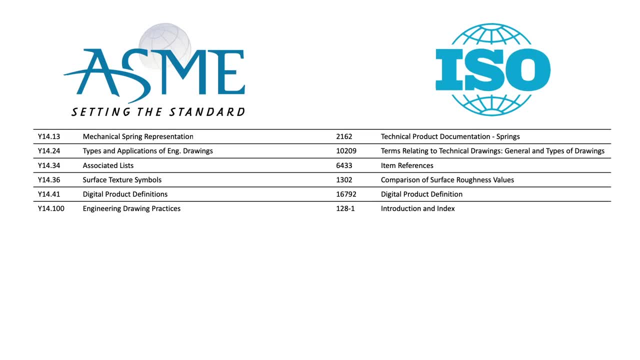 Engineers, which is the default in the United States, in which of Canada and Mexico. In the rest of the world, ISO standards are typically used. There are some minor differences between the standards, but a lot of the fundamental concepts we're covering in this video apply. 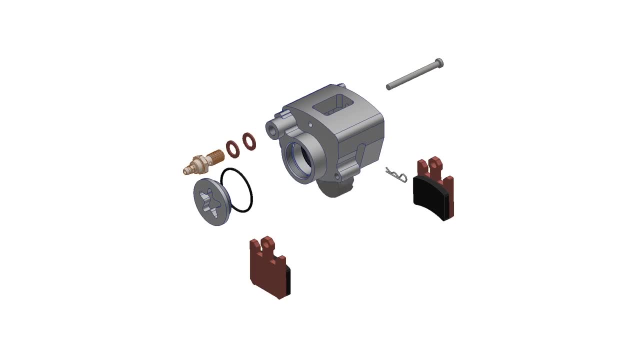 to either system. For the rest of this video, we're going to use this brake caliper assembly as an example. We'll highlight some rules, best practices and tips for both the detail and assembly drawings, but we're not going to show placing every dimension. 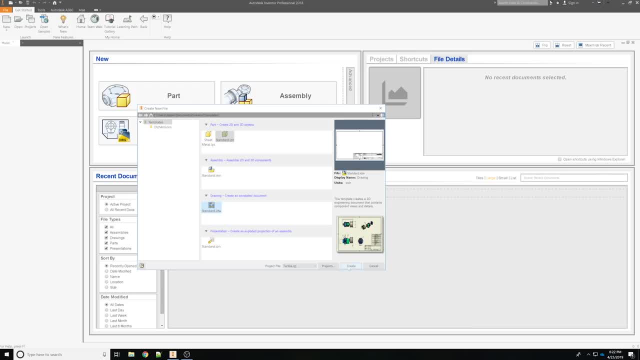 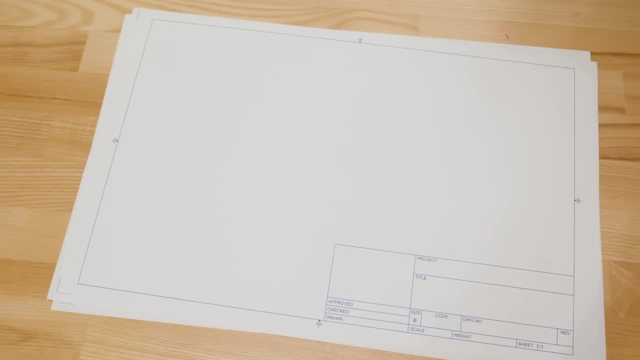 because that would make for a very tedious video. When making a drawing, you'll usually start with a template, which is typically the same for both detail and assembly prints. At the time of this video, the template that is built into Fusion 360 is not compliant with the ASME drawing standard. 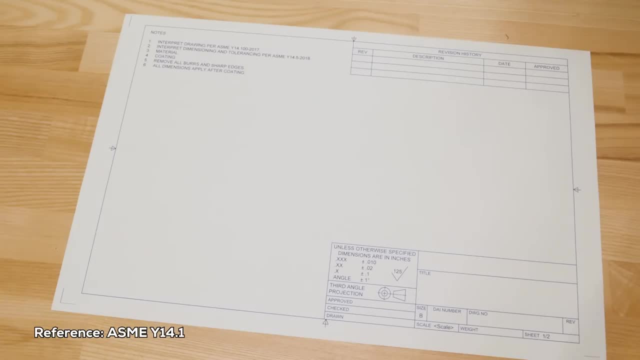 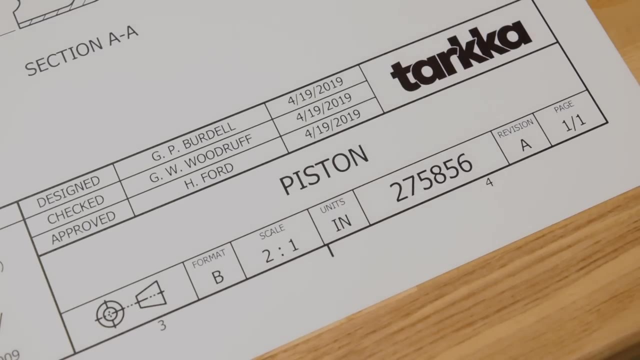 We've made our own standards-compliant template for Fusion 360,, which you can download from our website. The title block gives information about the company and people responsible for the design, as well as the drawing name, number and revision. It also specifies the sheet size. 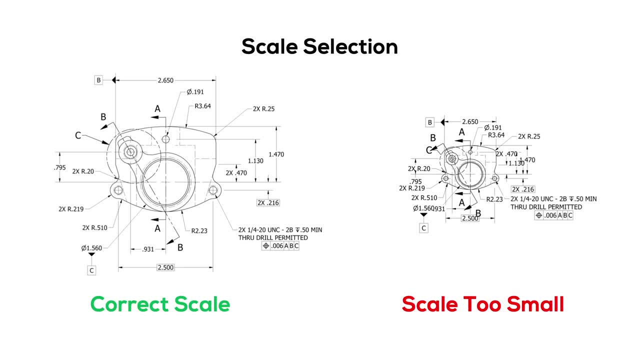 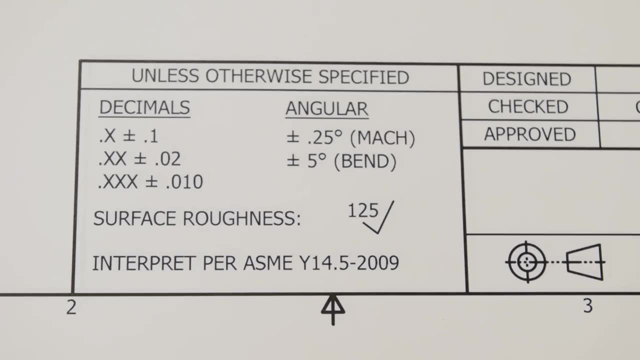 and primary scale, and you'll want to choose these so that you have enough room to place all the dimensions in each view. Within the title block there's also a list of blanket tolerances that apply when a dimension is given on the face of the drawing without an explicit 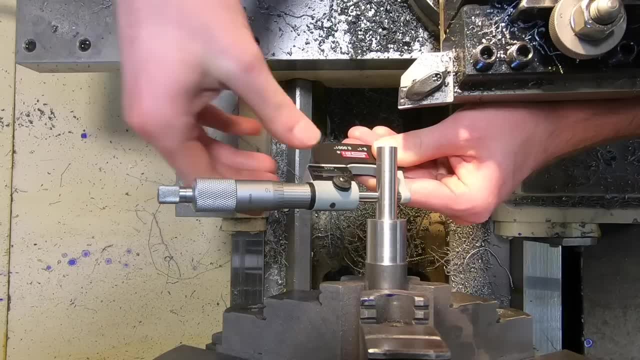 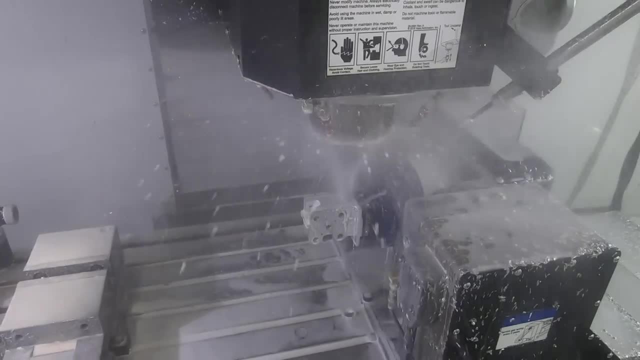 tolerance. A big problem we see with drawings are title block tolerances that are unreasonably tight. In the format we've provided, we tried to choose tolerances that are reasonable for most modern CNC machines, but you may want to increase these even more depending on the type of work you do. 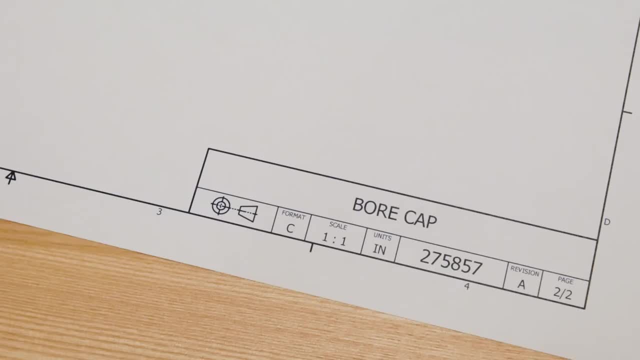 The title block is a very simple and easy-to-use tool that you can use to make your drawings. The title block on subsequent sheets of the same drawing usually contains less information and is called a continuation title block. The revision table shows when the drawing was changed. 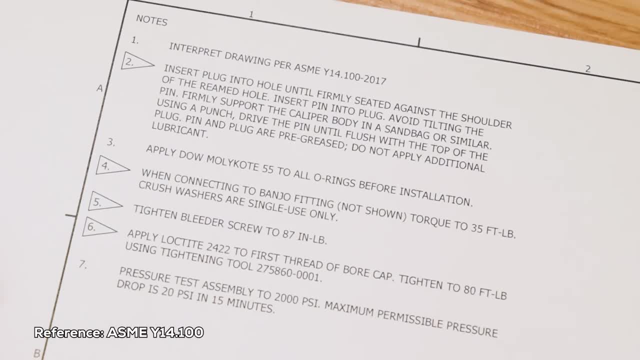 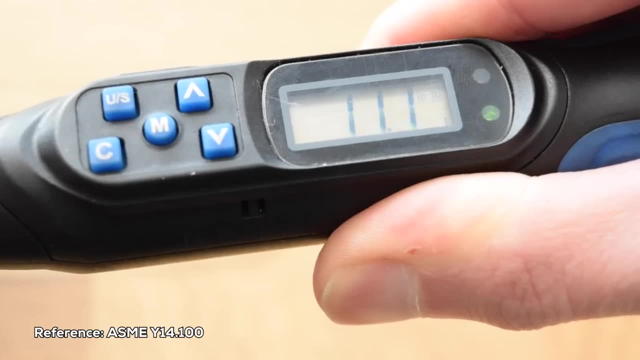 for what reason and by whom. The notes list provides information like the material and coding specifications, relevant standards needed to interpret the drawing, special instructions for manufacturing certain features and other information that can't be conveyed with a dimension. The border defines zones with letters and numbers that allow you to identify specific. 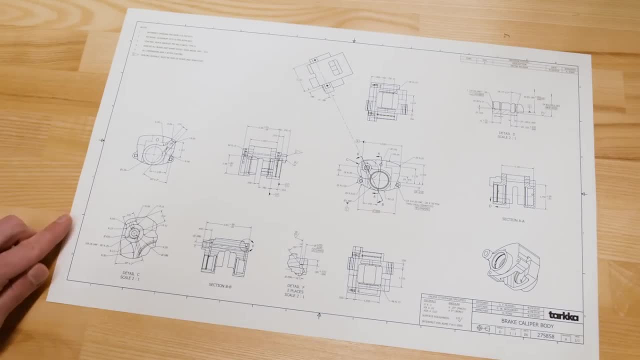 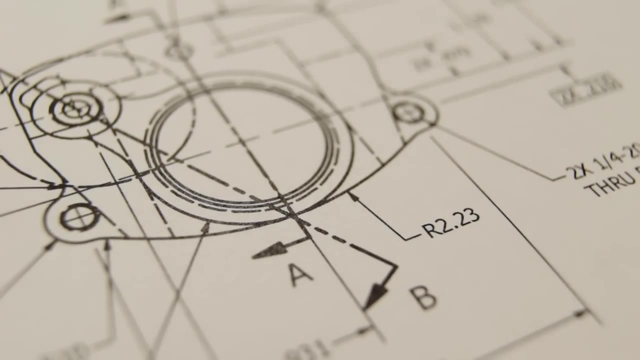 features with coordinates. This is really handy on big drawings, because you can say something like: change the 0.19 hole diameter in zone A7. And be able to jump right to it instead of having to scour the entire drawing to find something. 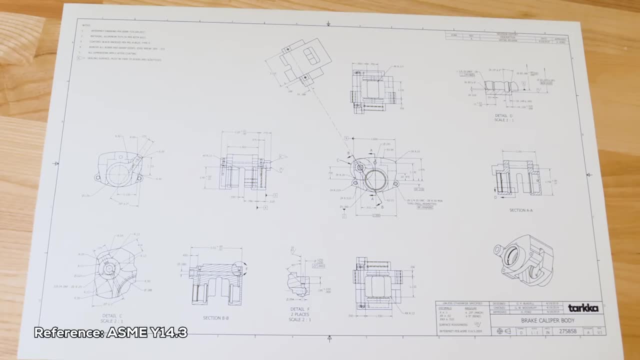 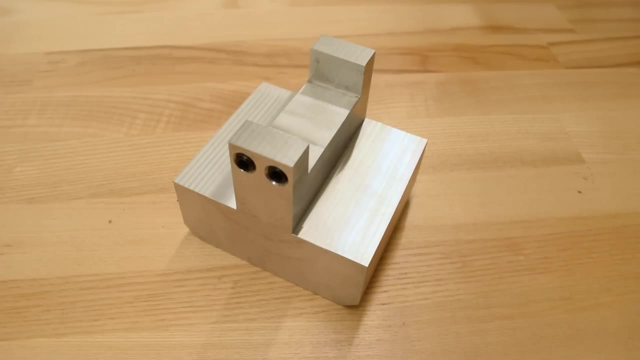 The face of the drawing will usually have two or more views and they must have a particular alignment to each other. We're going to switch to hand drafting for a second to talk about where this convention comes from. To draw this example part, we're going to choose a view to be our. 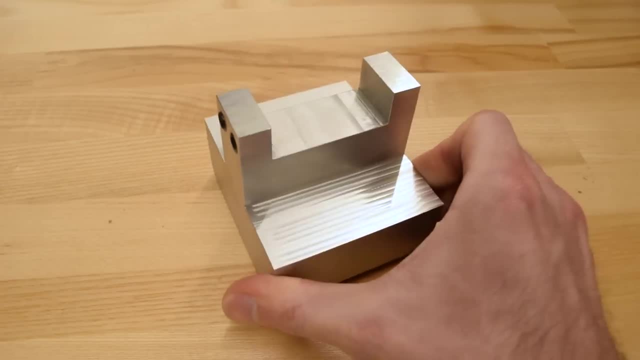 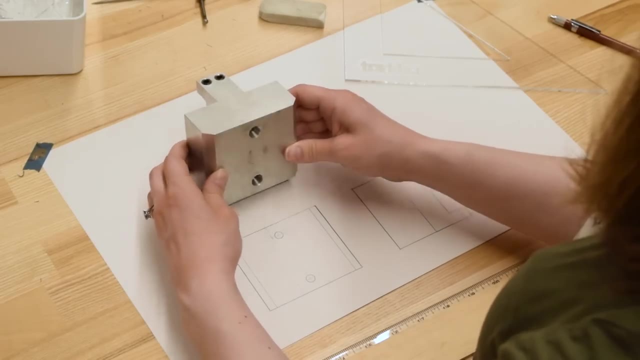 primary or front view, But there's other features of the part, like the larger tapped holes in the slot that can't be seen, so we need to create additional views around the front view that show them. To draw these projections, we have to imagine that we are rotating the part in space. 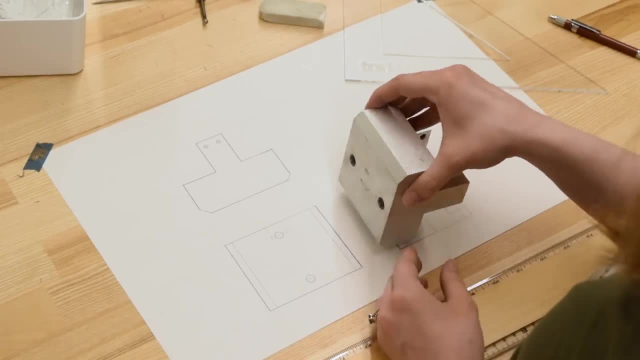 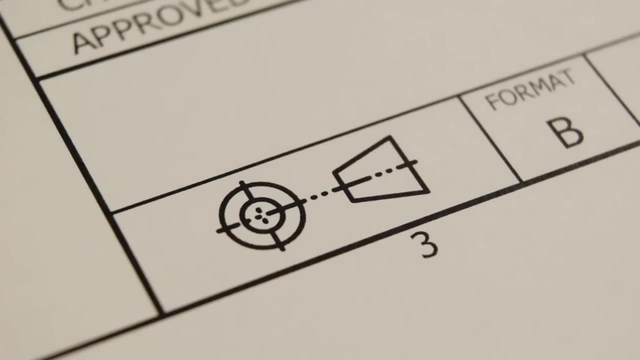 If you're making drawings in the United States, you would rotate the part in this direction. This is called third angle. To detail other views, you'll project the lines from your front view to define the features. You need to make it clear in the title block which convention you are using. 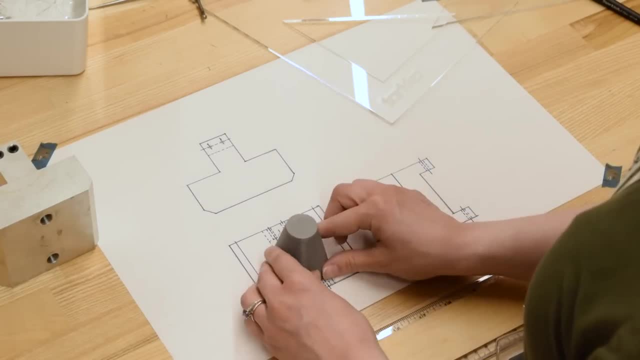 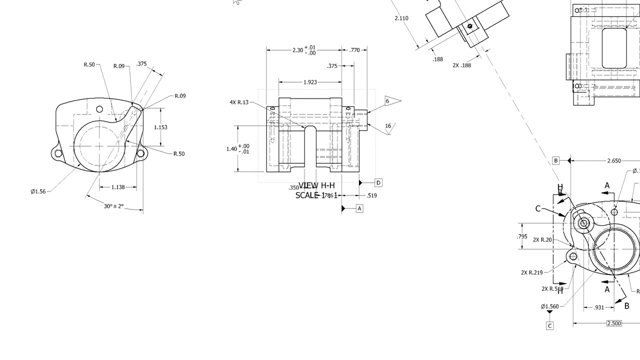 And that's what the cone symbol is for. 3D CAD can create problems because it allows you to very easily break the alignment and place a view wherever you want. You should really avoid this, because the person reading the drawing will use the orientation of the views to reconstruct the part in 3D and breaking the 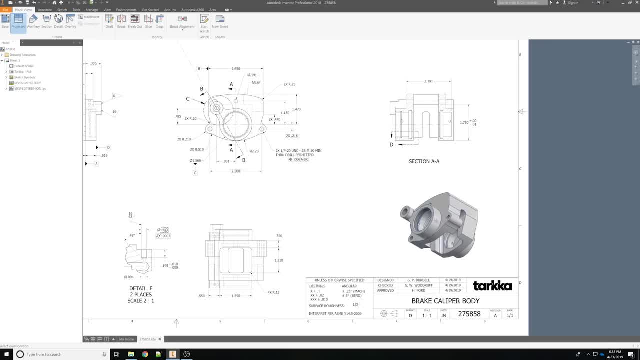 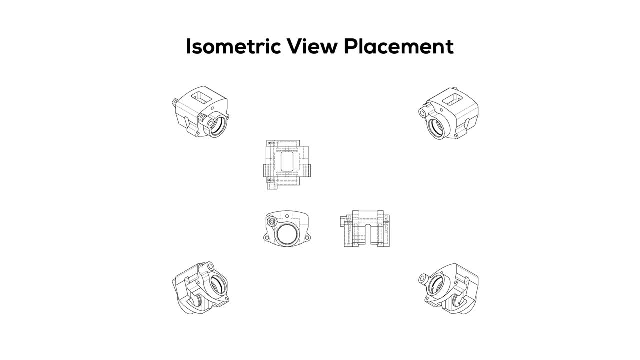 the standard alignment makes this process much more confusing. It's also a great idea to drop an isometric view to help clarify things. Isometric views don't have to be strictly aligned to the orthographic views, but you should draw them in the correct corner for the orientation you want to show. You can put: 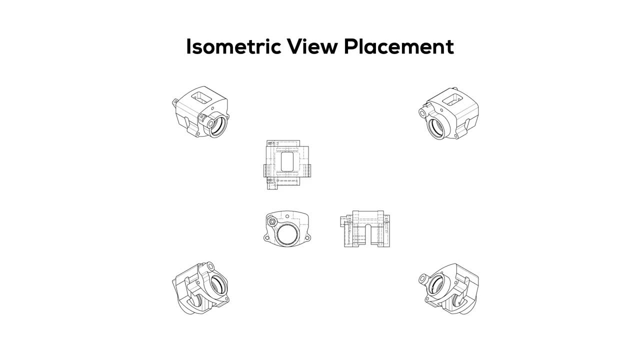 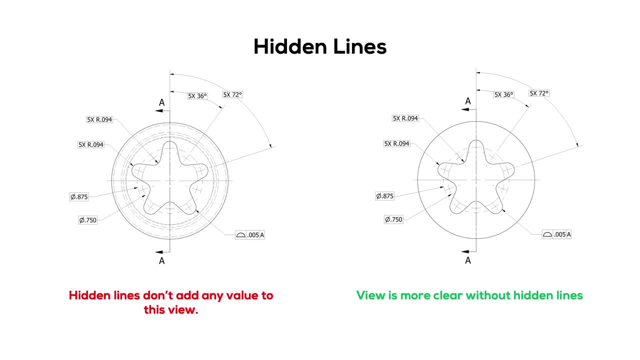 notes in an isometric, but you don't put any dimensions, since the features don't appear in their true size or shape. You'll usually want to show hidden lines to help depict the internal features of a part. However, having lots of hidden, 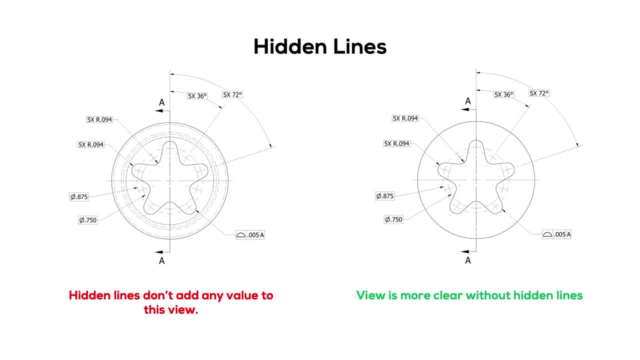 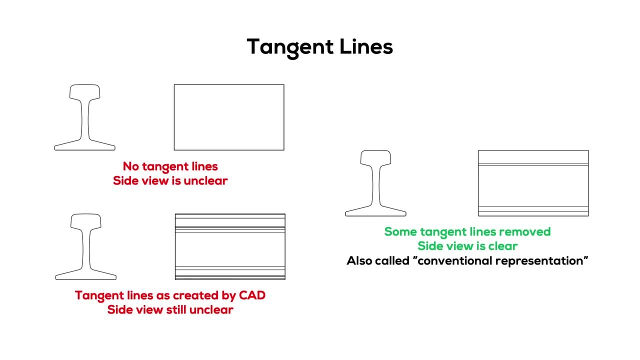 lines can sometimes add confusion, so you can omit some lines for clarity. This is really a case-by-case thing, and your primary objective should be to make the drawing as clear as possible. The same is true of tangent lines. You will usually omit them in orthographic views, but sometimes they're needed to make the 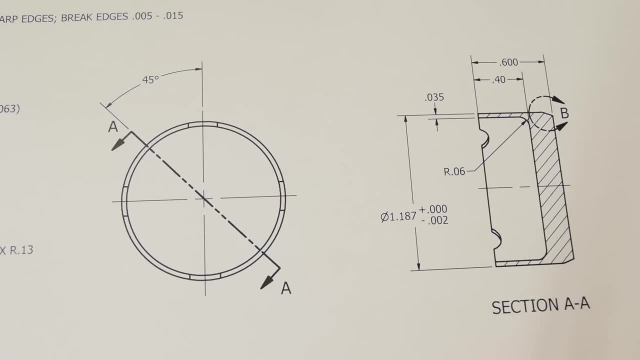 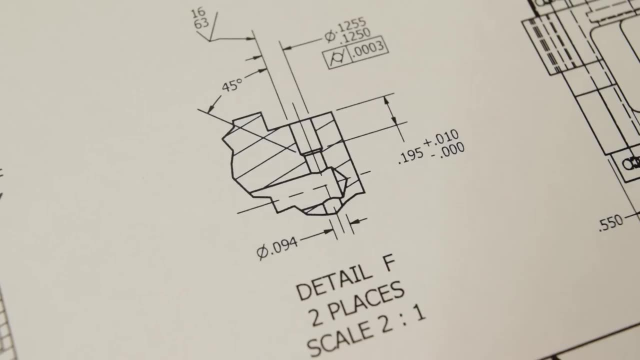 view recognizable. You should also avoid dimensioning to hidden lines, so you will often need to create section views to dimension internal features. Smaller features often need to be shown at a larger scale and detailed views can help you do this. With your views arranged, you can start adding dimensions When. 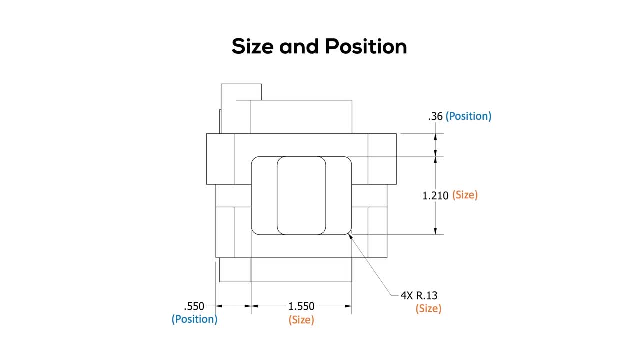 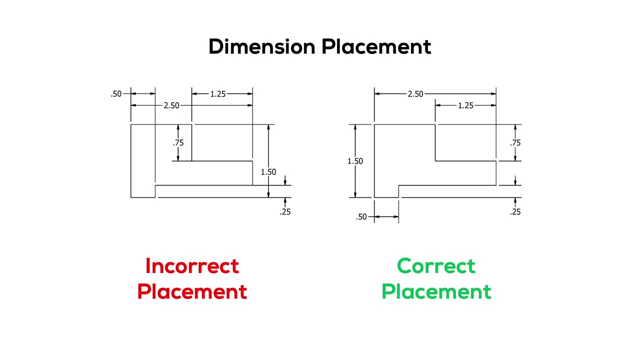 placing dimensions. you need to fully define the size and position of every feature, and this is where new engineers typically struggle the most, so be sure to check out the reference sheet on our website. The general rule is that dimensions should be placed outside of the view You are not allowed to cross. 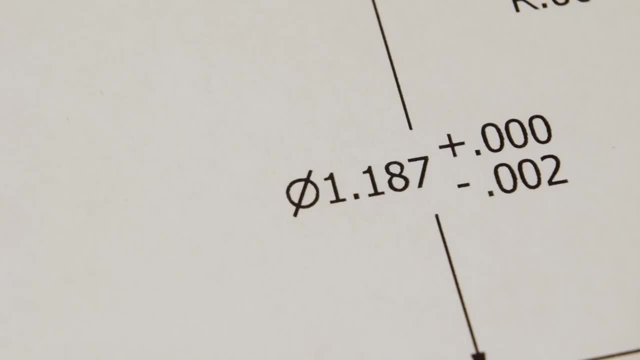 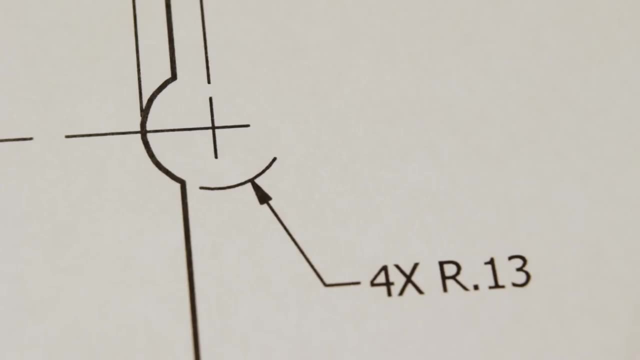 the dimension lines, with either extension lines or leaders. Round features and arcs greater than 180 degrees should be dimensioned according to their diameter, and a diameter symbol will precede the dimension. Arcs less than 180 degrees, like fillets, should be dimensioned by their radius and a letter R should. 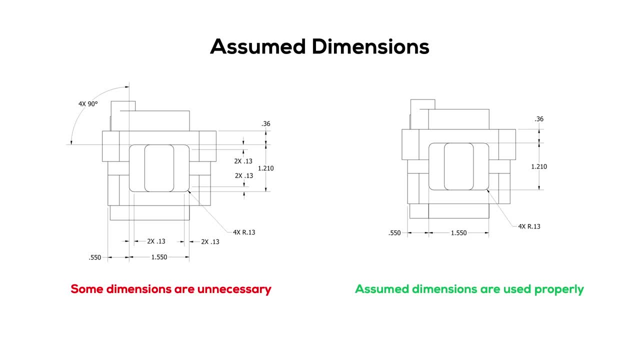 precede the dimension. There are some features you don't have to explicitly define. If two edges meet at a 90 degree angle, it's just assumed to be 90 degrees. you don't need to place an angle dimension. Similarly, edges that appear to be tangent. 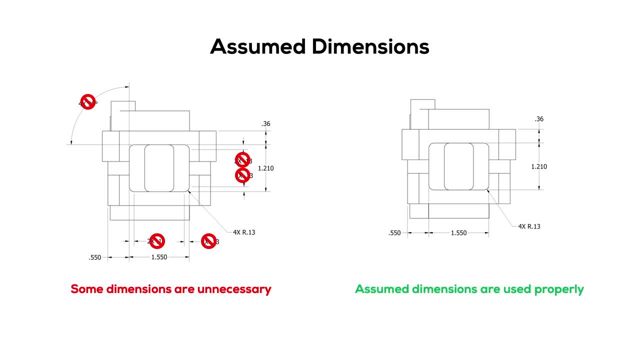 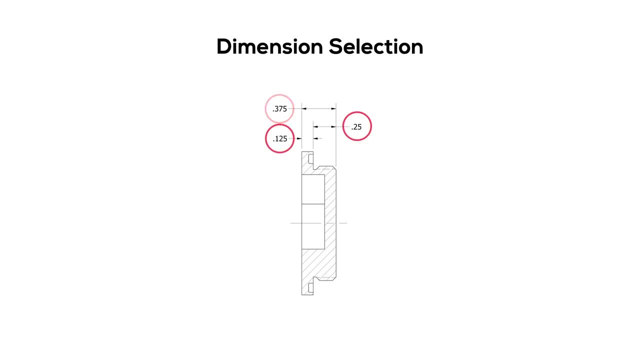 like fillets, are assumed to be tangent. You cannot have multiple dimensions that conflict with each other. For example, this view of the borecap has an overall length dimension, as well as these dimensions that define the thread length and flange thickness. These dimensions conflict, and one of the three 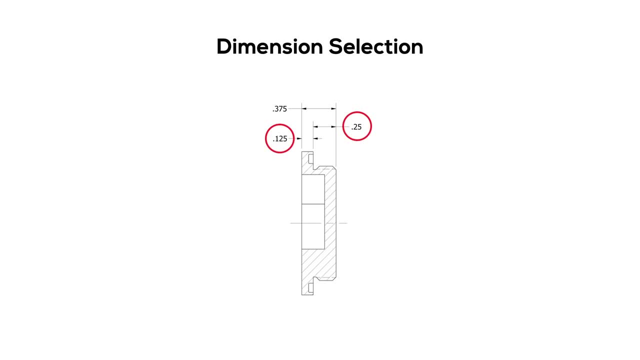 is redundant To minimize the tolerance stack. it's best to dimension it with these two. but having the overall length is helpful and we want to show it on the drawing. To resolve the conflict we can. We can place parentheses around the overall length, denoting it as a reference dimension. 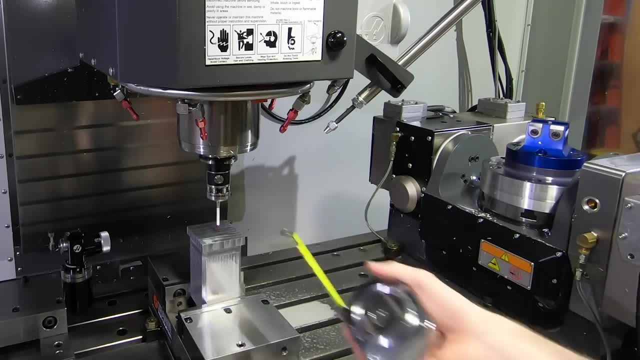 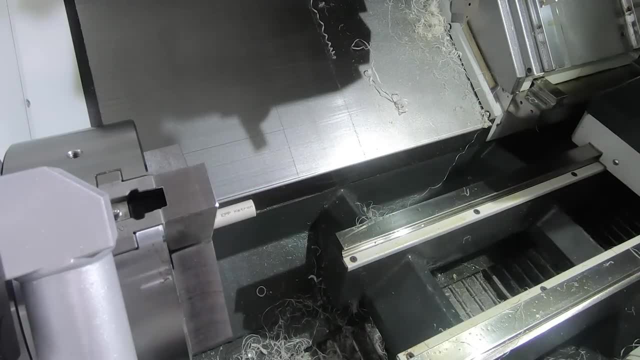 This means it doesn't control the part in any way and is simply for informational purposes. It can be very helpful to provide reference dimensions that show the overall size of parts, so you can easily see the size of stock needed to make it. Threads are called out with a note that specifies the size standard and usually the tolerance. 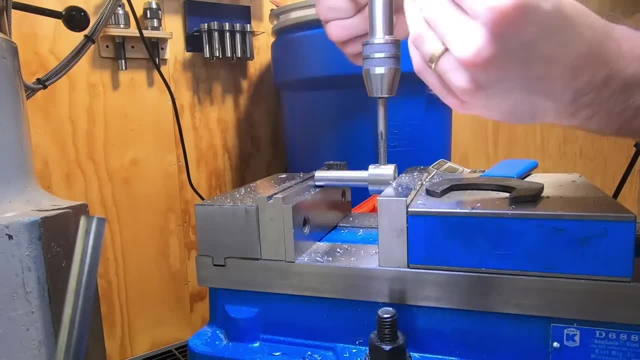 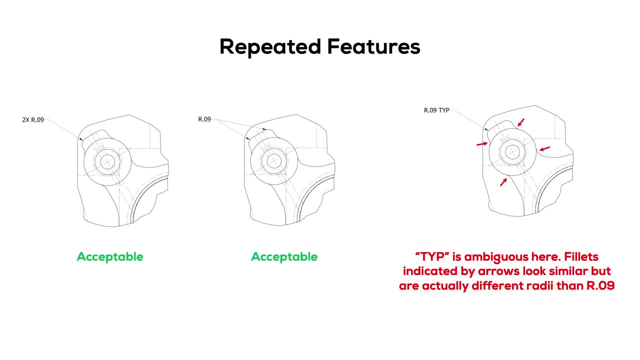 class. You can also specify the depth in the note or with a dimension in a view. Many times you'll have multiple instances of the same feature, like these fillets. You can use a note like 2x to indicate this, or multiple leaders. 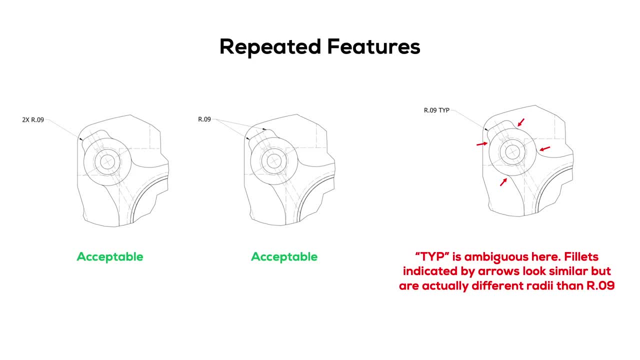 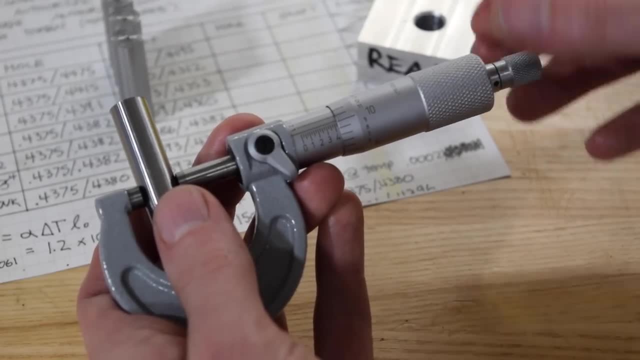 Sometimes people will put TYP for typical, but you should avoid doing this because it can be extremely confusing when there are multiple features that look similar but are really different. Critical features in your drawing will often require tighter tolerances than what is stated in the title block. 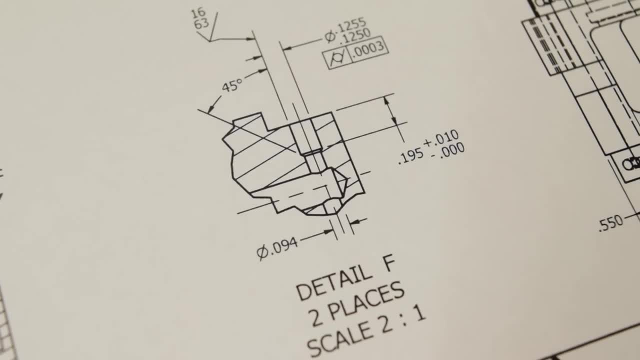 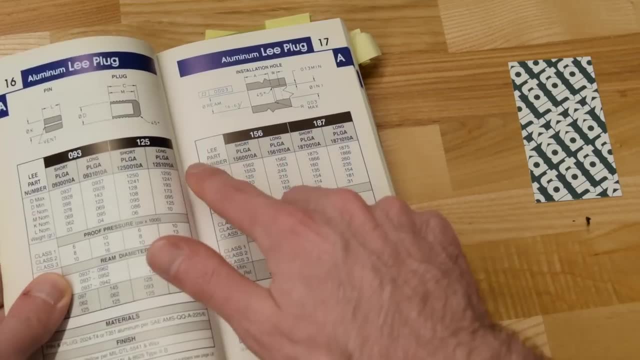 A lot of times the tolerances will be provided to you by somebody else. For example, this hole holds a special type of hydraulic plug from the Lee Company. Their technical references call out the dimensions and tolerances, so we can just copy that onto our drawing. 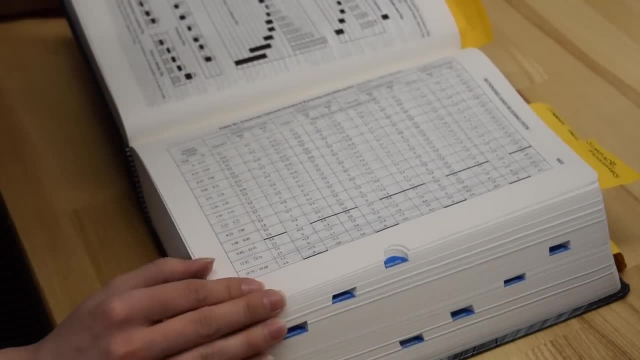 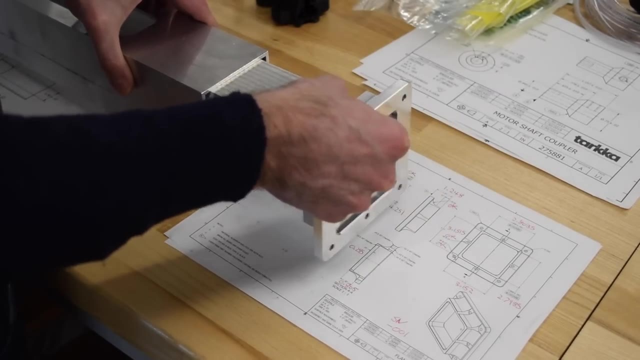 In an earlier video we talked about how to use design tables to set the tolerances for the fit you need between components. For more complicated interfaces, you can use a technique called geometric dimensioning and tolerancing. GD&T is fairly complicated and we're going to have to make multiple videos just to cover. 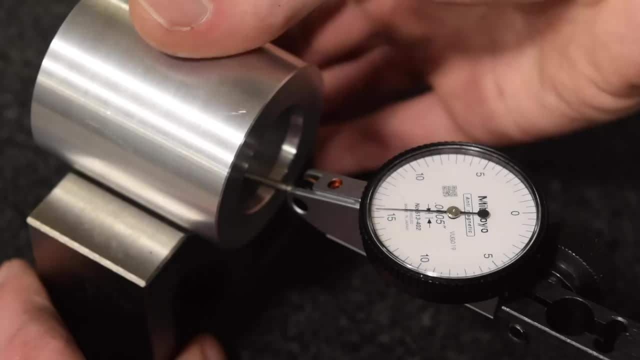 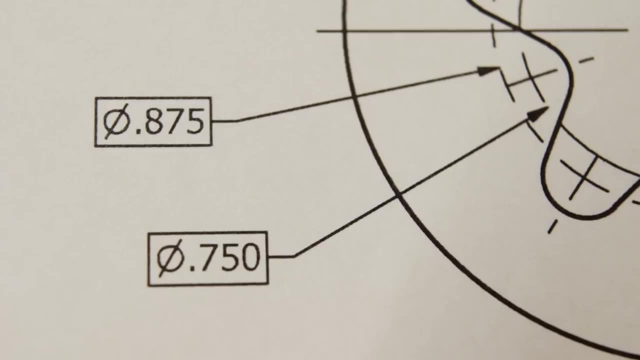 all the nuances, but until then, here's the elevator pitch. GD&T gives you a way to describe the functional requirements of features by controlling things like flatness, perpendicularity, position and runout. When using GD&T to control a feature, the locating dimensions are typically enclosed. 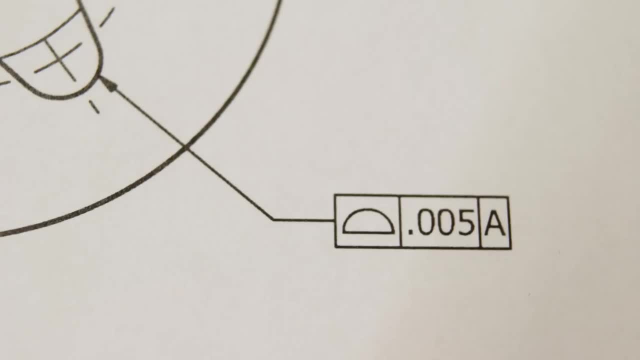 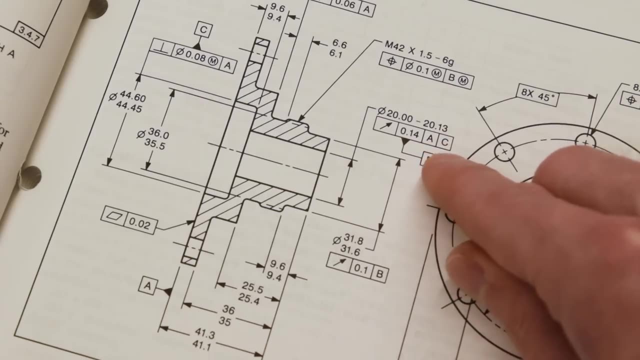 with a box to indicate that they are basic or theoretically exact. The feature is controlled by a special node called a feature control frame, which may also reference other features as datums. If it sounds complicated now, don't worry, because we're going to break it all down. 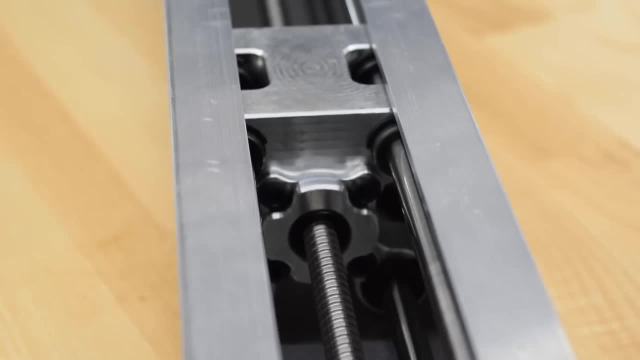 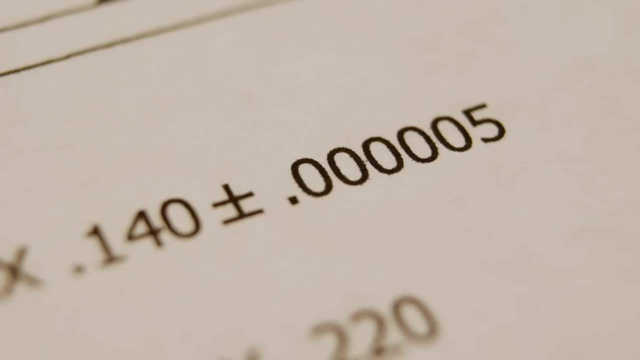 into much simpler terms in future videos. The important thing we want to emphasize is that there is a systematic way to calculate what every single tolerance should be to achieve the intended functionality. It's terrible practice to put an arbitrarily tight tolerance on a dimension, but it's 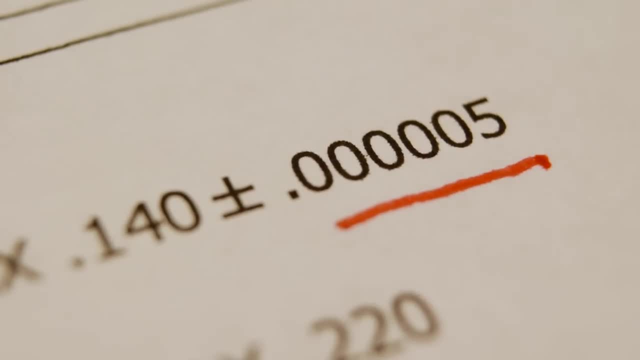 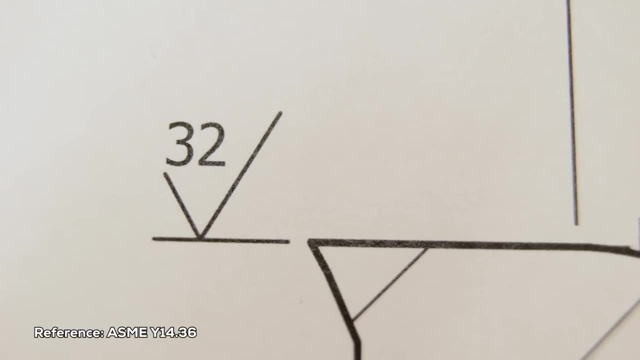 a great way to calculate what every single tolerance should be to achieve the intended functionality. You will often need to specify surface finishes. in locations where you have a seal, There is a special symbol to do this. The number indicates the root mean square height of the surface in micro-inches and 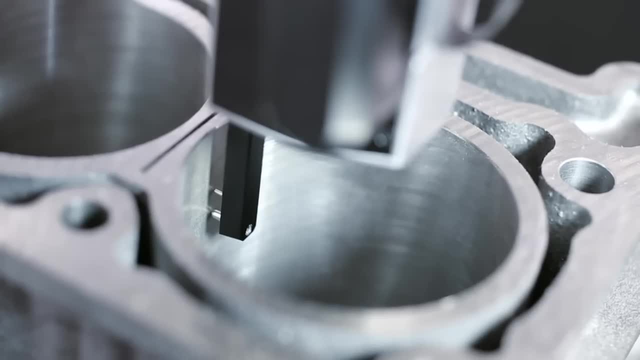 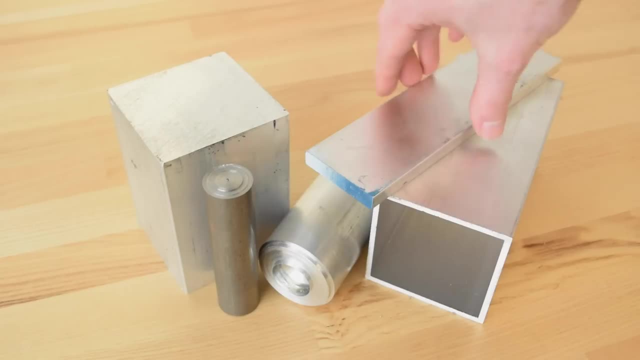 this is inspected with a special type of instrument called a profilometer. Notes are critically important for clarifying the drawing and fully defining the part. A lot of notes will apply to the entire part or drawing. For example, you can use notes to specify things like materials or coatings. 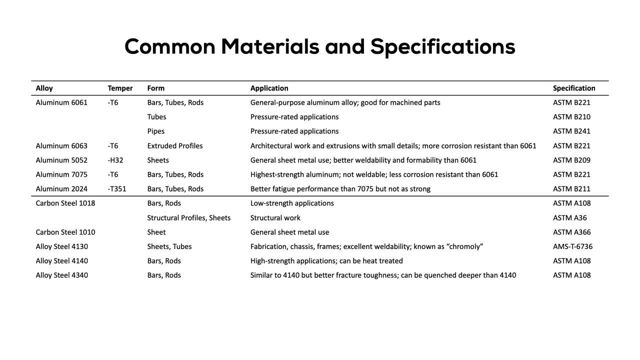 When listing material, it's critical to specify the alloy heat treat and material. This is important because it's important to specify the alloy heat treat and material. It's important to specify the alloy heat treat and material. Just saying something like 316L stainless is not enough, because this particular stainless 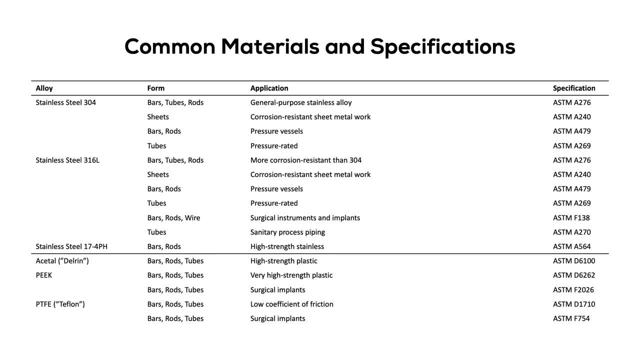 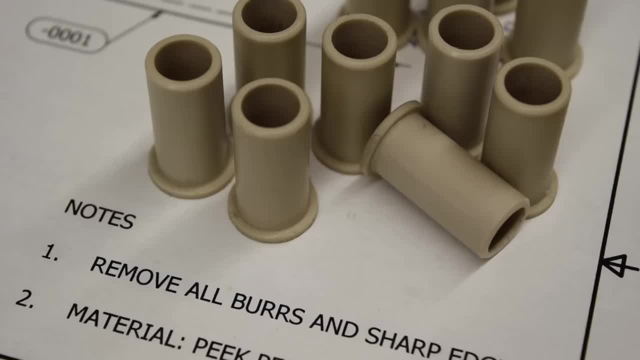 alloy can be made for normal industrial applications or an ultra-high purity and cleanliness for pharmaceutical and biomedical applications. You need to list a specification to clarify which version you need. You should not use notes to specify things like quantity, delivery date or payment terms. 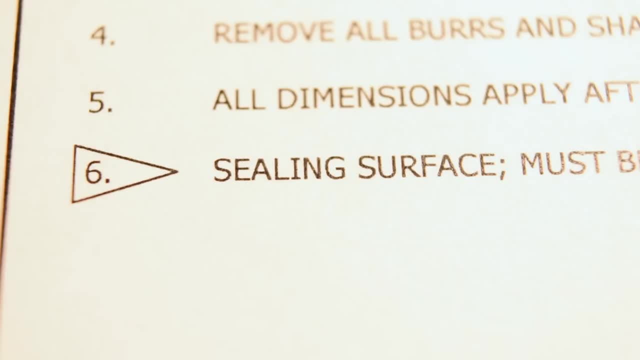 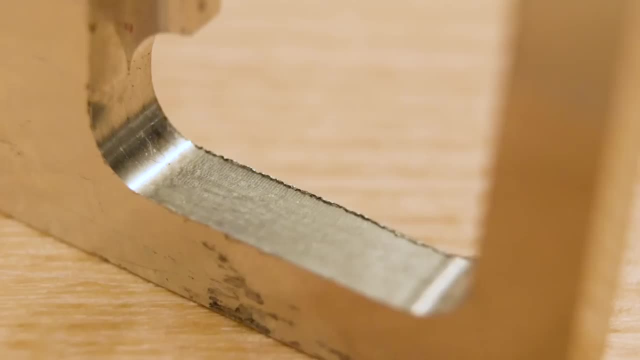 This information will be listed in the request for quote and purchase order. Other notes will only apply to a specific feature. These are often called flag notes because a little flag symbol is sometimes used. You typically don't want to have sharp edges on any finished parts because it presents. 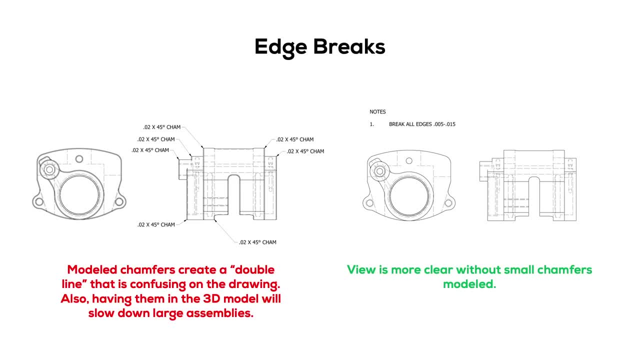 a safety concern and burrs can interfere with components fitting together. If all you want is an edge break, best practice is not to model or dimension small chamfers or fillets. Instead, you can use a general note asking the manufacturer to remove burrs and sharp. 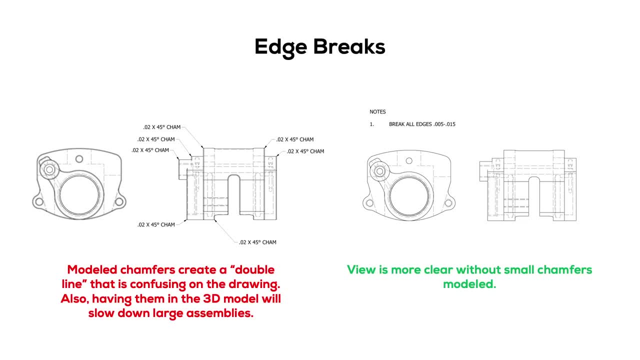 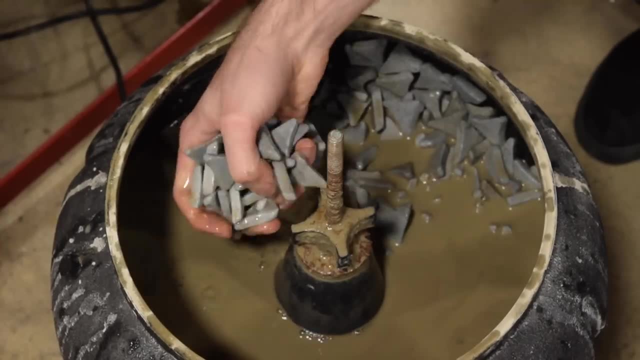 edges and perhaps only supply a loose range for the size of the edge break. If you use a note like this, you are giving them the option to deburr on the machine using a hand tool- grinder, bead, blast or a vibratory finishing machine. but if you place dimensions,